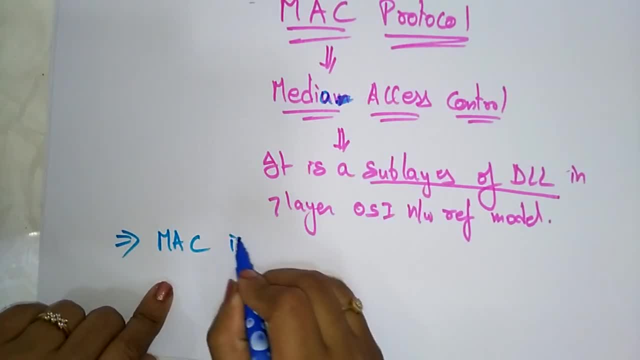 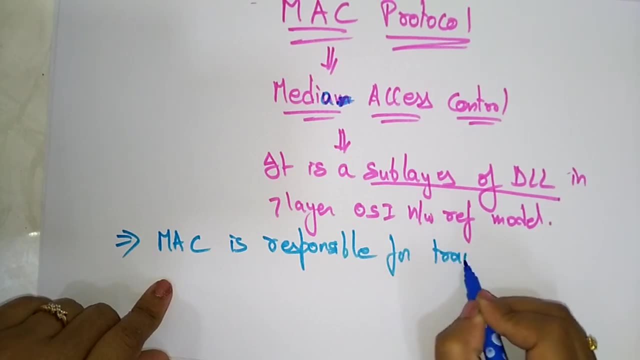 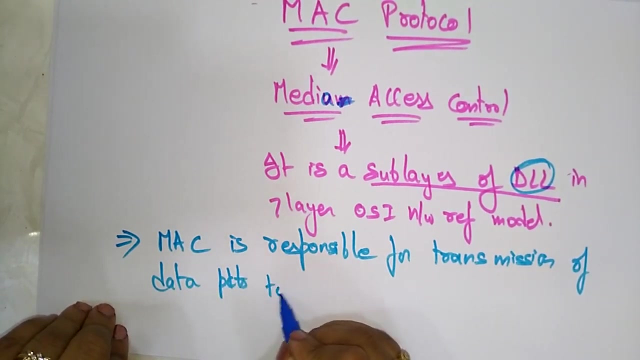 so the media access control is responsible for transmission of what transmission of data packets we are talking? it is a sub-layer of data link layer, so it is responsible for transmission of data packets, data packets to and from the network, to and from network interface card. 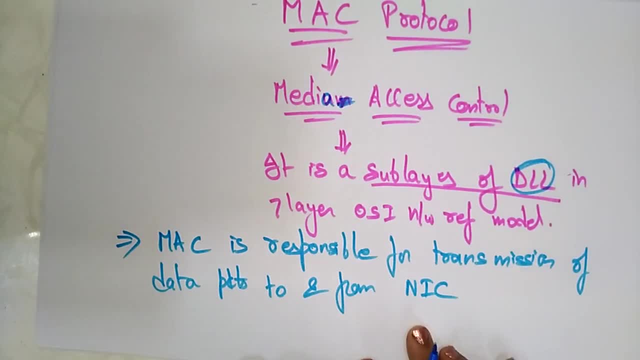 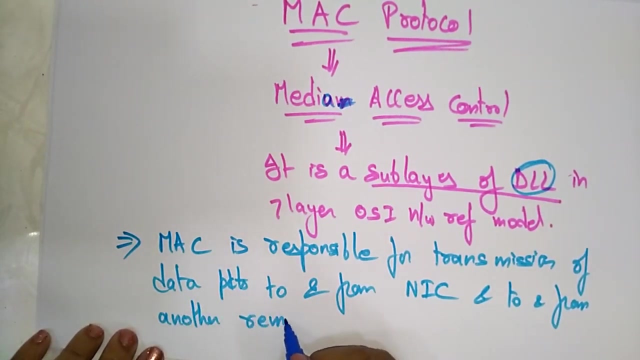 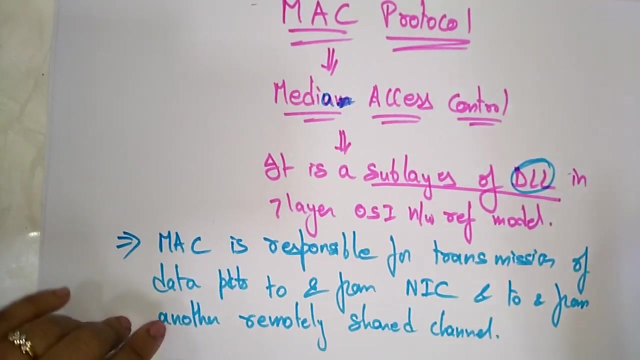 to and from network interface interface card and to and from another remotely shared channel. to and from another remotely shared channel. it's a simple thing: the MAC media access control, which is a sub-layer of data link layer. 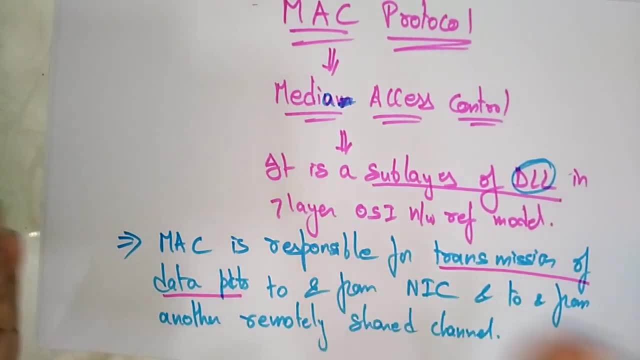 is responsible for transmission of data packets. it is going to transmit the data packets. this MAC protocol is transmitting the data packets to and from the network interface card and also to and from another remotely shared channels, and if any channel is there shared channel, it is also sending the data packets that from those remote channels also. okay now, what is the main aim of this? 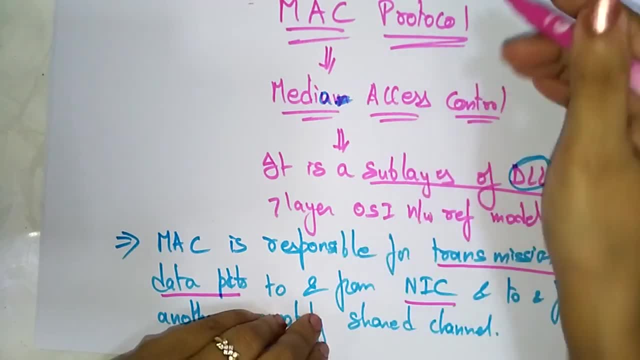 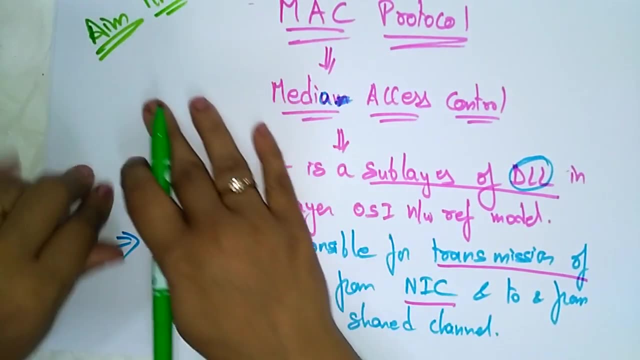 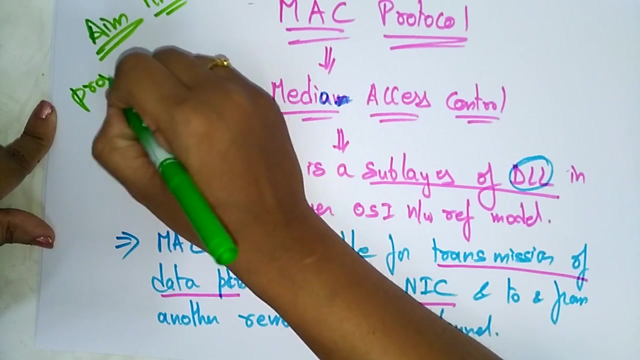 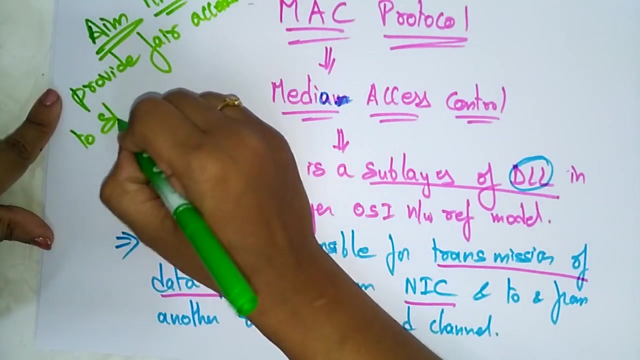 media access control. the main aim here is- let me write the aim of this MAC. the main aim of the media access control is it provide the fair access. provide fair access to shared broadcast, to shared broadcast radio channels. 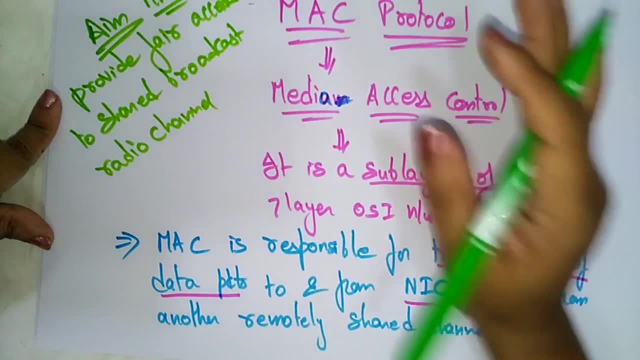 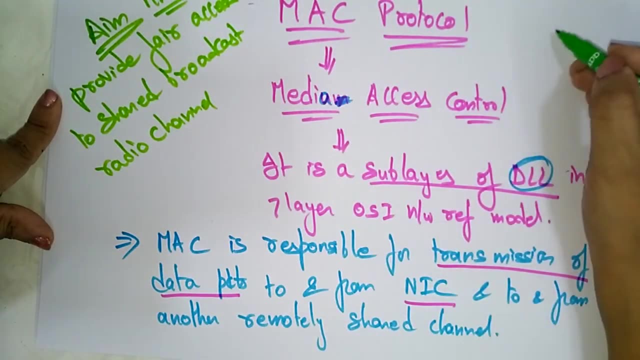 we are. the MAC itself is a media access control, a media accessing control, so it provides a fair access to the shared broadcast radio channels. suppose the radio channels will be there if you want to send the packets to and from the radio channels. 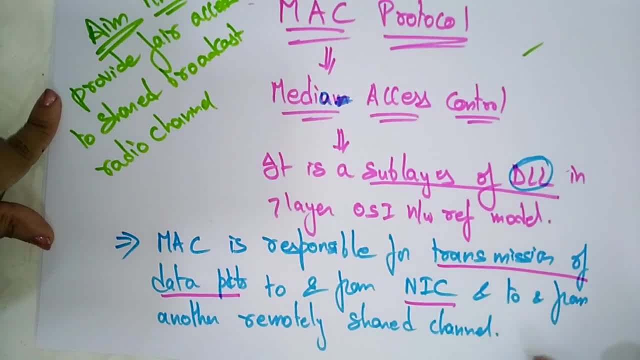 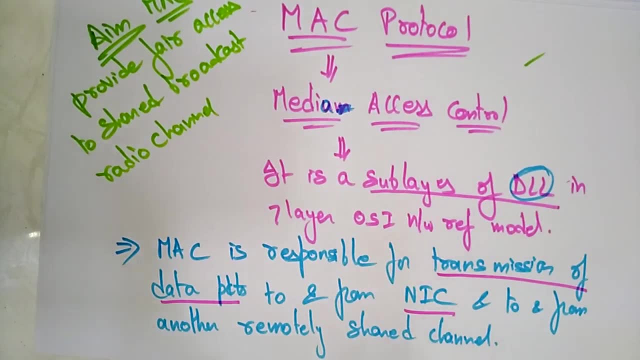 this MAC protocol is providing a fair access to those shared broadcast channels, radio channels. so this is just an introduction of this MAC protocol. a MAC is a media access control which is a sub-layer of the data link layer in the seven OSA reference models.